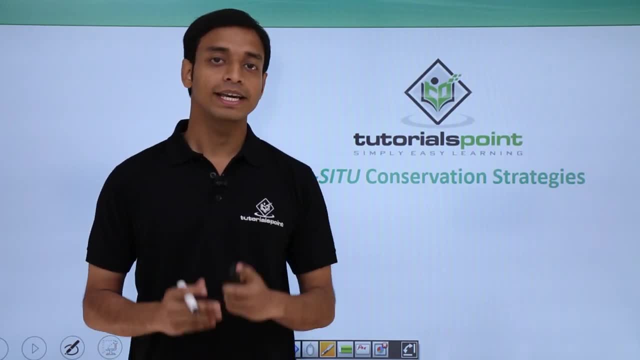 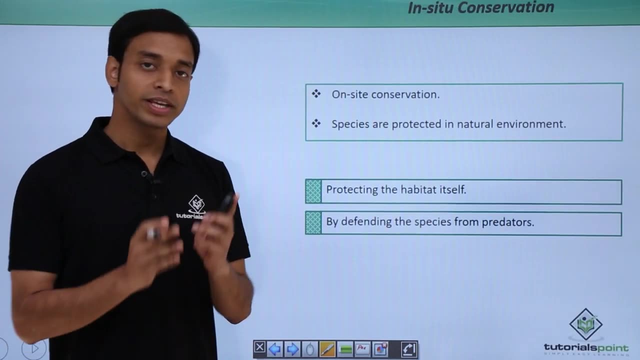 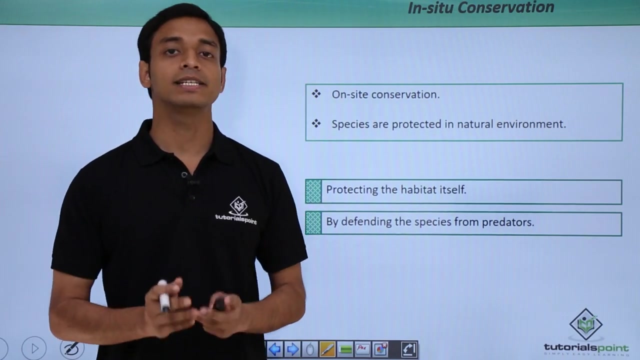 Hello everyone, Welcome to Tutorials Point. In this video we are going to talk about in-situ conservation strategies. So what is in-situ conservation? In-situ means on-site conservation, Conservation which is performed at the natural environment, That is, species like. 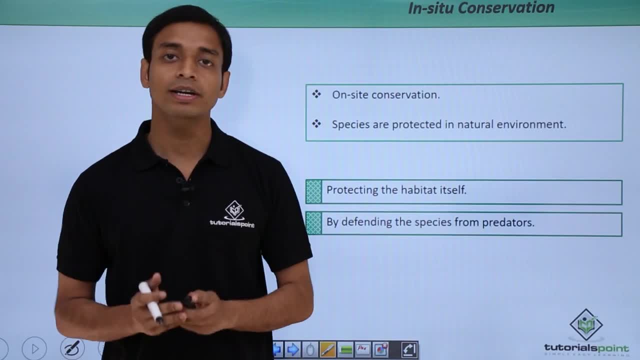 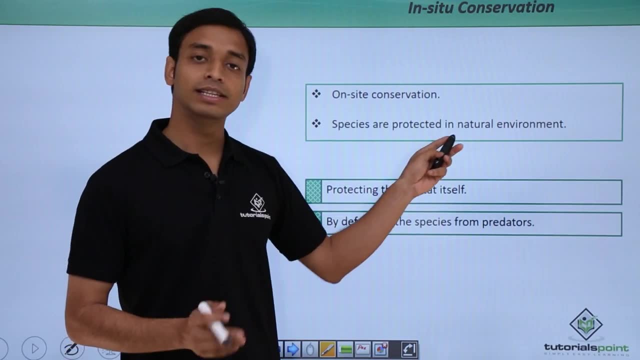 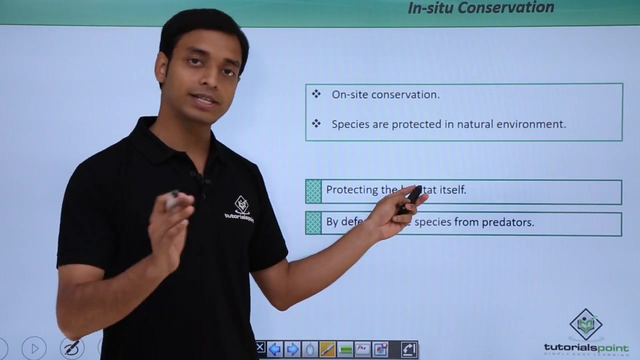 plants and animals are not taken out from the natural environment, and hence the conservation is performed in this type of method. Now here, species are protected in the natural environment. Now this can be done in two ways. First of all, it can be done by protecting the habitat itself. 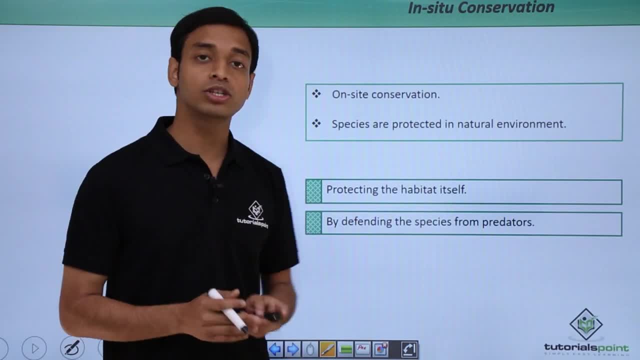 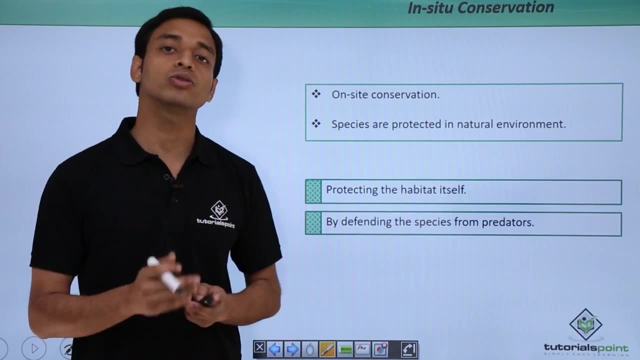 or else we can also do by defending the species from its predators or the. we are trying to control the danger end of this particular species we are trying to conserve. Now let us look into the different types or different strategies of in-situ conservation that we are trying. 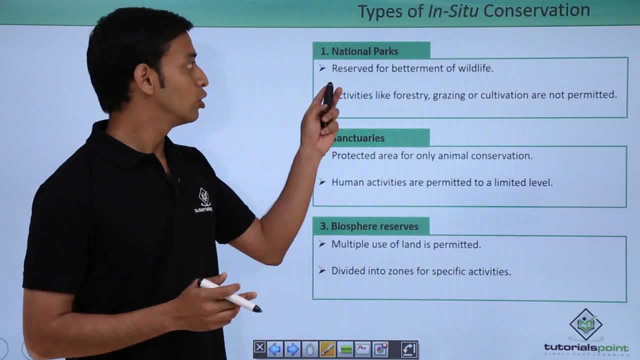 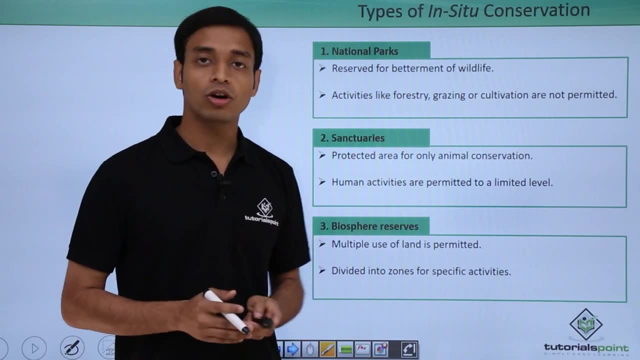 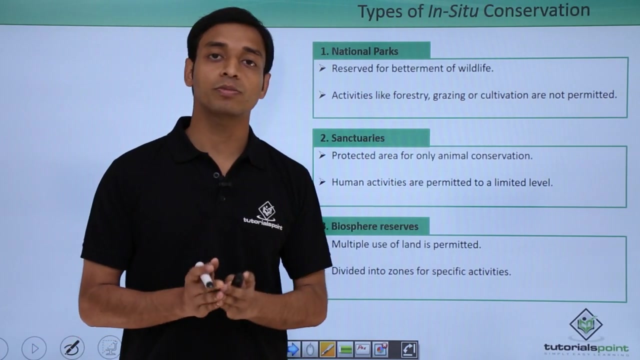 tried to adopt. The first one we have tried to develop is known as national parks. So what are these? These are actually specifically reserved for the betterment of wildlife. Here, no human activities like forestry, grazing, cultivation, are not permitted at all. So this is a fully 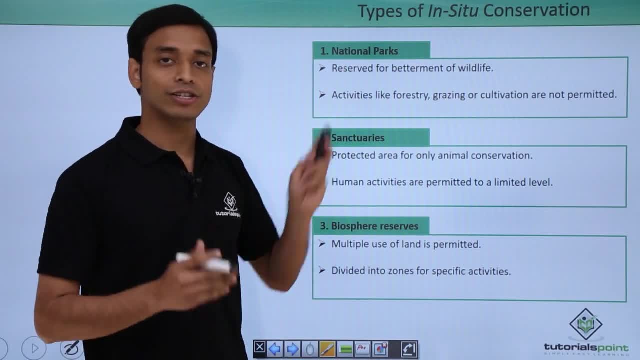 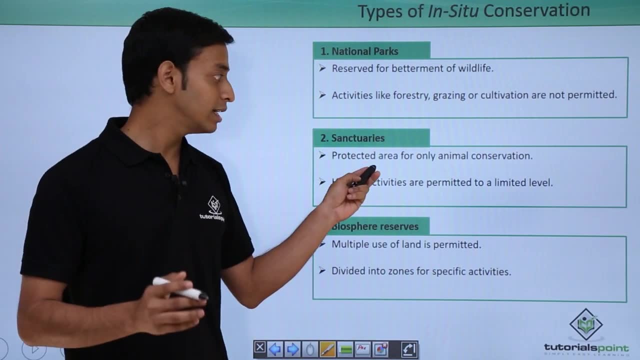 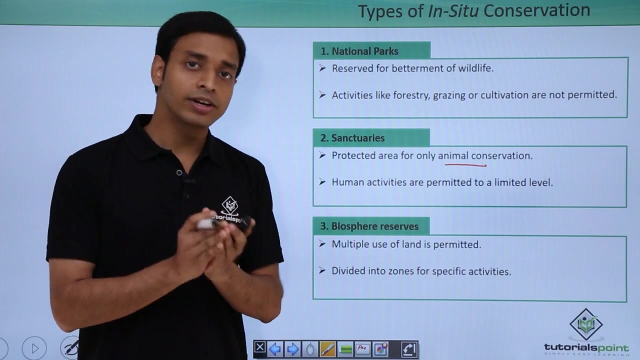 protected environment. So this is a type of this is known as national parks. The next type is known as sanctuaries. So what are these? These are also protected areas, but specifically for animal conservation. Now we try to protect the animals over here. Here it's a bit different from the 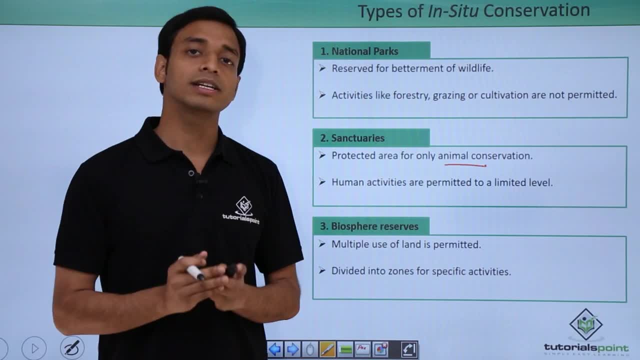 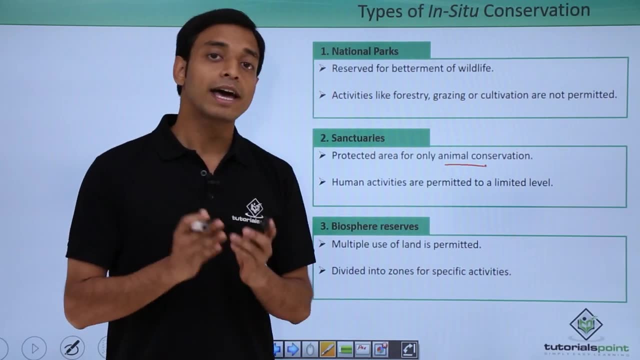 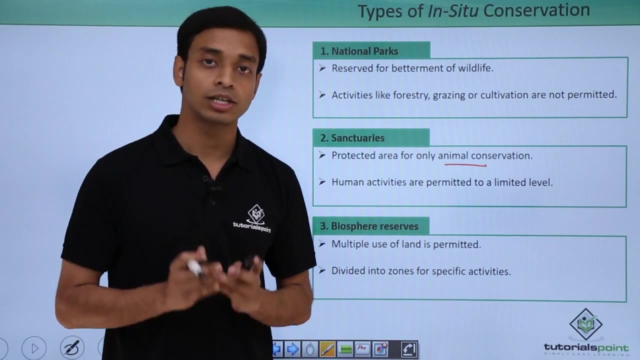 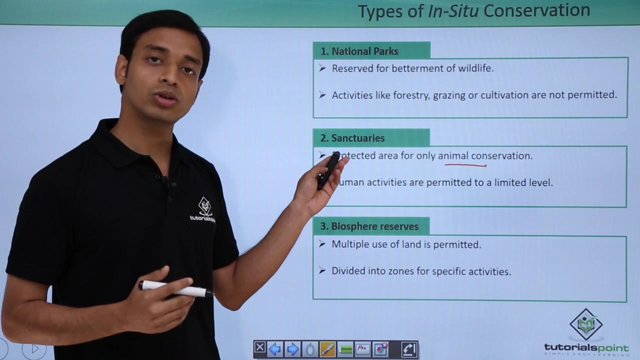 national parks because to some extent some type of human activities are allowed, Human activities like collection of timber, collection of forest products and also some private ownership rights are also given. but the important point is to a limited extent, To a extent till which it is not hampering the natural ecological balance. So these are types. 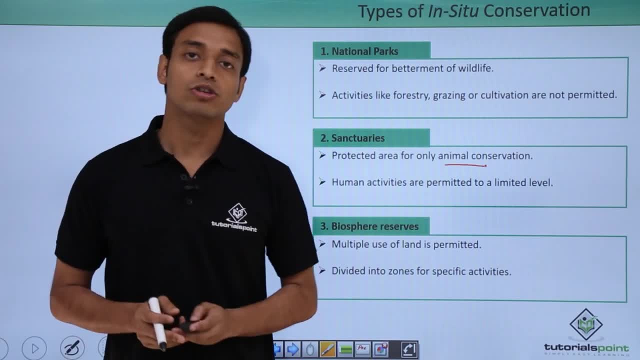 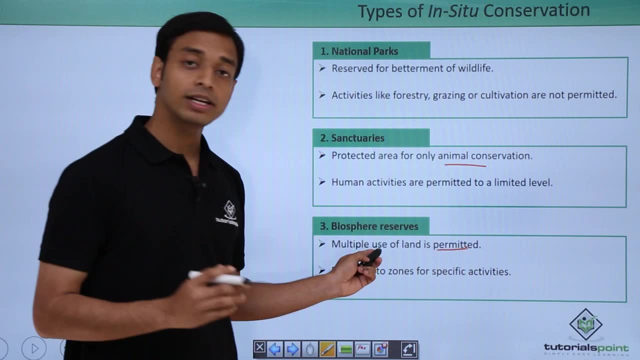 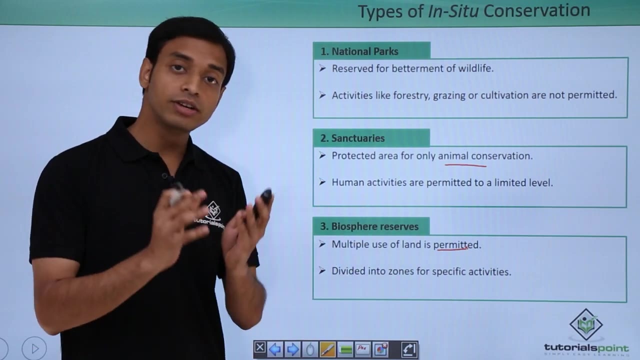 are known as sanctuaries. The third type is known as biosphere reserve. This is a different type in which multiple use of land is permitted, Unlike these two. here use of land, or multiple use of land, is permitted. Now, how it is done: It is divided into different zones for different purpose.